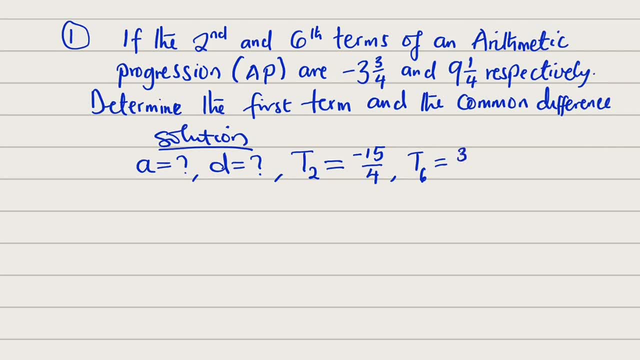 which is thirty seven divided by four. All right, now, this is our data. We are given second term from the question, and second term can be obtained by adding common difference to the first term, And first term is A plus the common difference, which is D, which we can now simplify to. 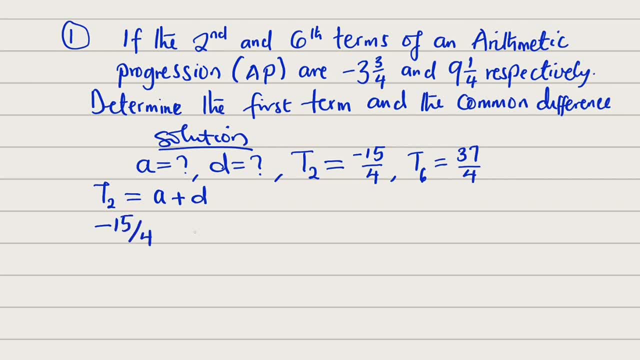 negative. fifteen over four equals A plus D. This is our first equation. We can form an other equation, which is equation two. We have seen that term number six can be of ten by adding five D to the first term. A plus five D is said to be the sixth term, And D6 is thirty seven divided by four. 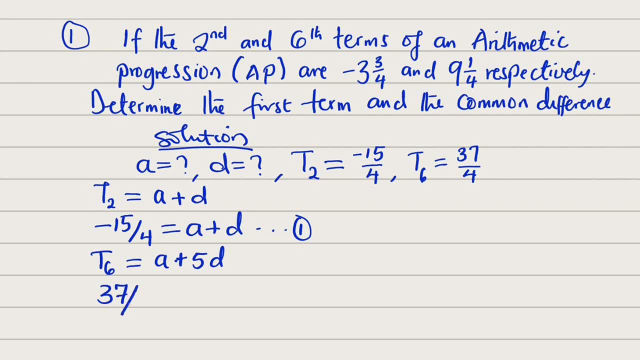 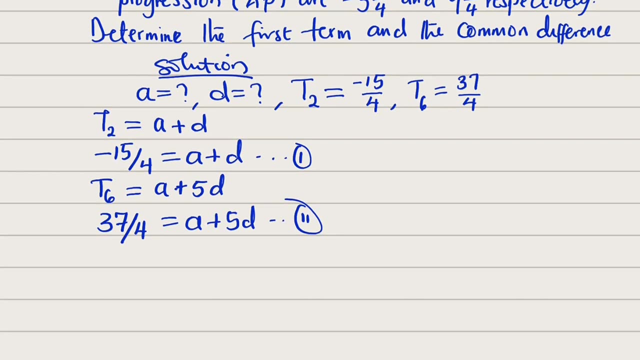 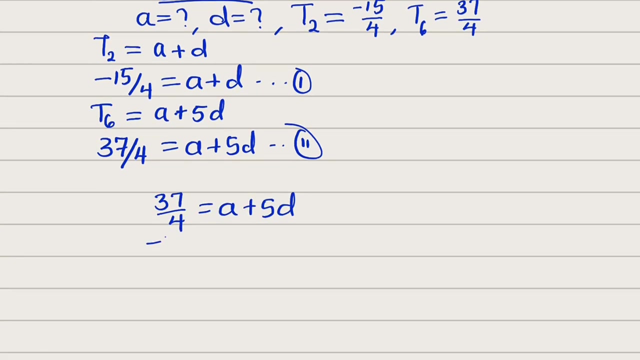 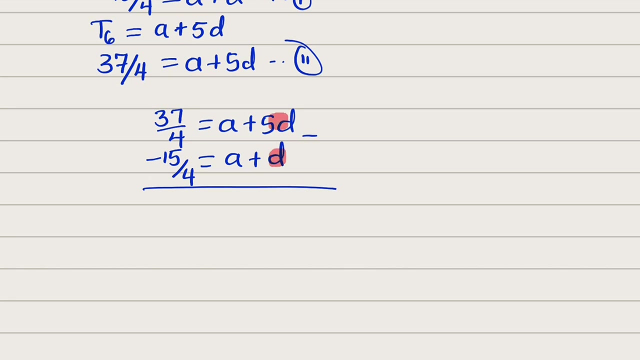 So thirty seven divided by four is equal to A plus five D, And this is our equation number two. All right, now let us say equation two minus equation one, to solve them simultaneously From the right hand side. five D, D minus D is four D. 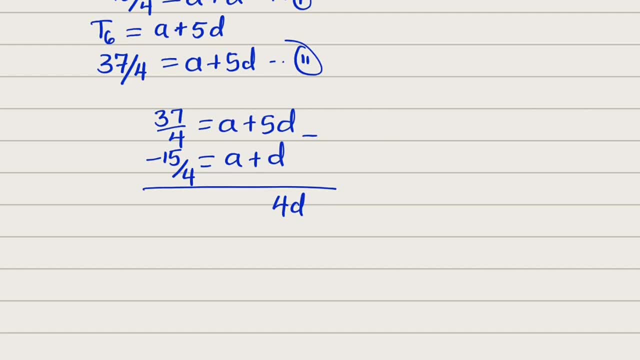 A minus A is zero. so we have only equality sign there. On the left hand side you can see we have common denominator four, four. Since we have common denominator, we are allowed to add or subtract denominators, But we have a negative sign which is going to transform this to positive sign. 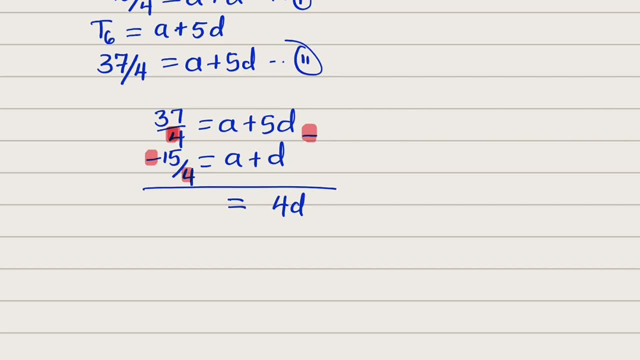 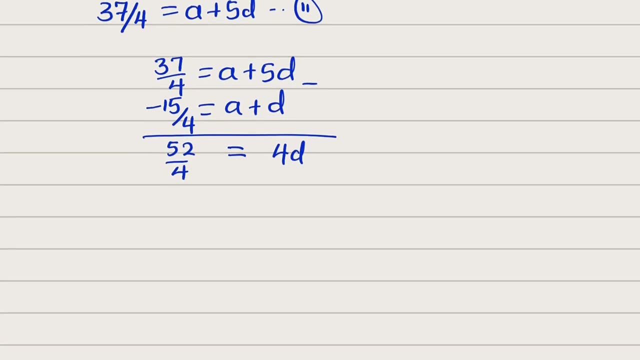 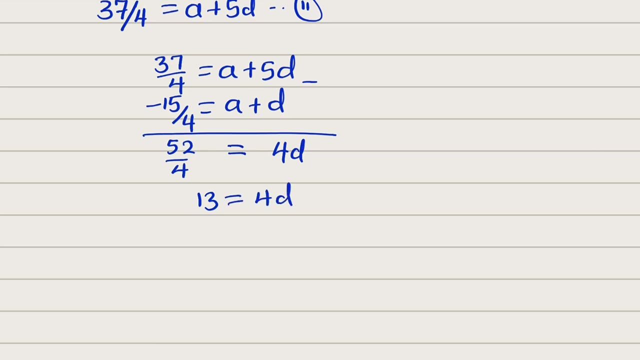 So instead we can say 37 plus 15, which is 52, so we have 52 divided by 4. 52 divided by 4 is 13, so we have 13 equals 4d. remember, d is our common difference. to find it, we can divide both sides by the. 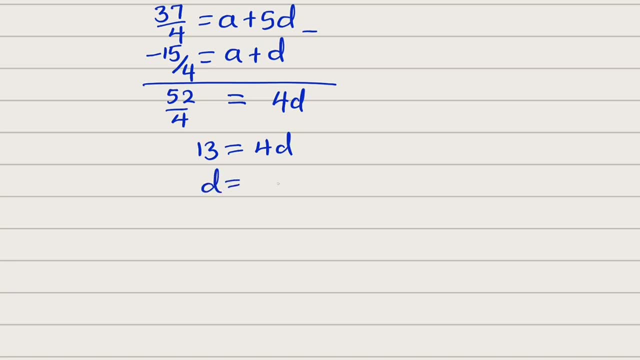 coefficient of d, which is 4. finally, d is equal to 13 over 4, or you can write it in mixed number three: whole number, 1 over 4. so now let us use this information to find the first term, which is a. we can even use this equation right here, so let me use that equation. 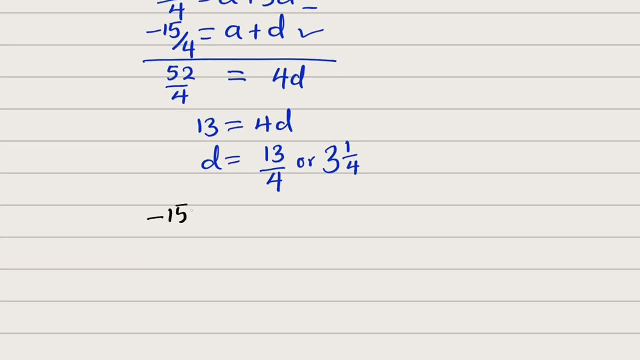 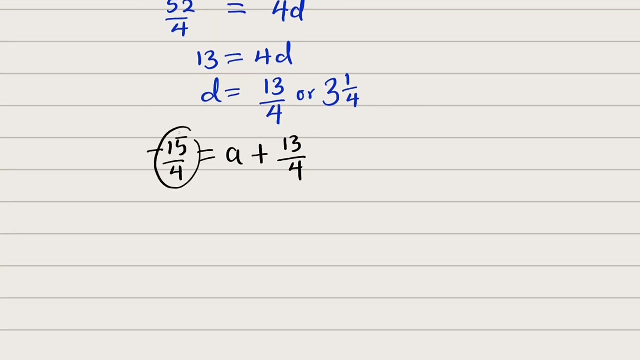 negative. 15 over 4 equals a plus d, but d is 13 over 4. let us multiply each term by 4 to clear the fraction from the left hand side. if multiplied by 4, we have only negative. 15 equals a. multiplied by 4 is 4a plus 13 over 4. multiplied by 4 is 13. 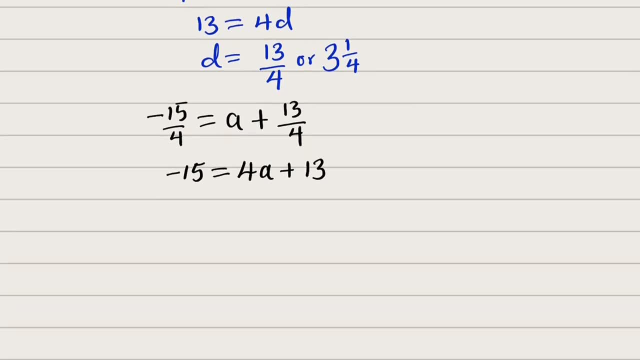 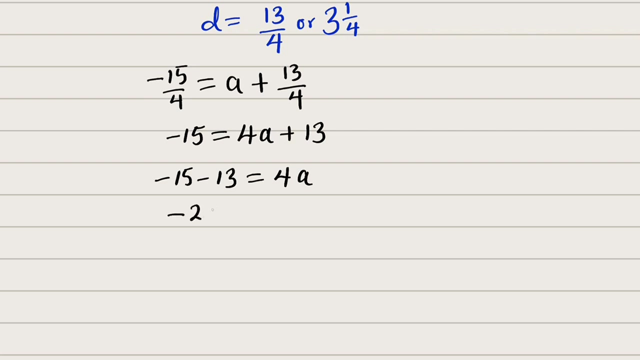 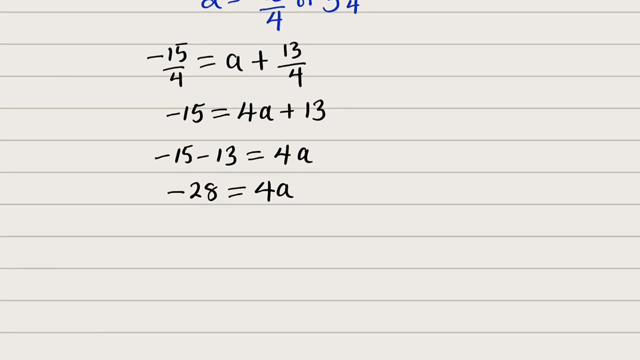 let us take 13. to the left, it becomes negative 15. we have negative 15, negative 13, and to the right we have 4a. to the left, we have negative 28 and to the right we have 4a. we are looking for a. therefore, now we can divide both sides by the. 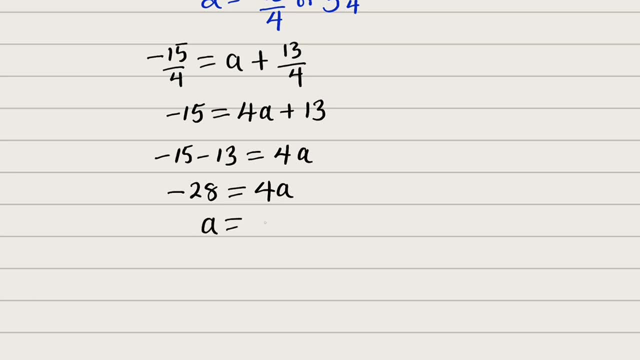 coefficient of a, which is 4. finally, a is equal to negative 28 divided by 4, and a is equal to negative 7, so we can see that a is negative 7 and d is 13 over 4, or 3, 1 over 4. 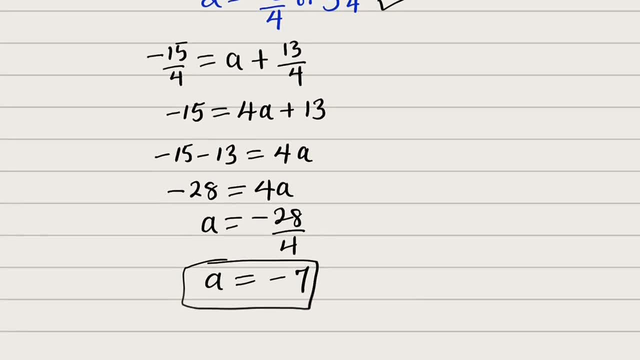 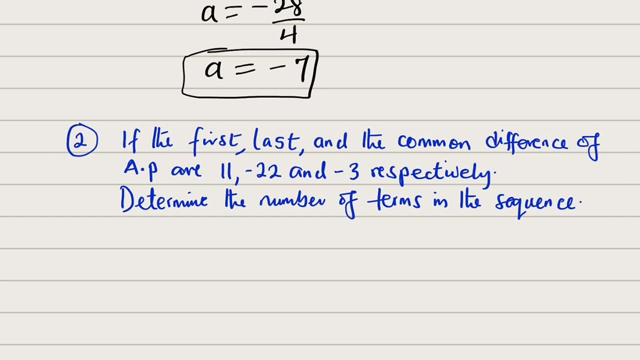 so now let us move on to the second question. so here is our second question, which says: if the first, last and the common difference of an arithmetic progression sequence are 11, negative 22 and negative 3 respectively, this implies that first term is 11, last term is negative 22 and the common difference is negative 3.. 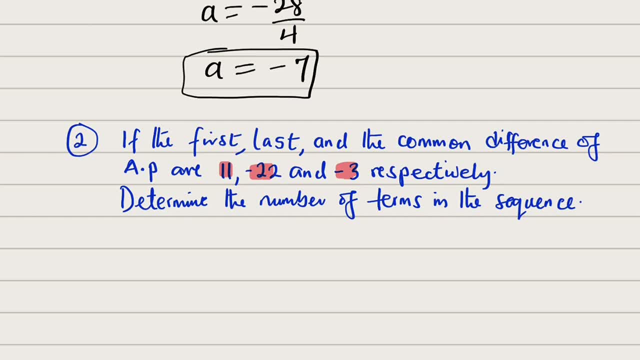 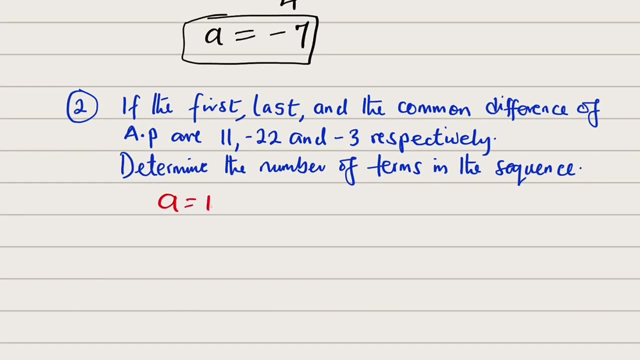 we are asked to determine the number of times in this sequence. first of all, let us write our data. we are given a as 11. we are also given the last term as negative: 12, 22.. We are equally given the constant common difference as negative, 3. But we 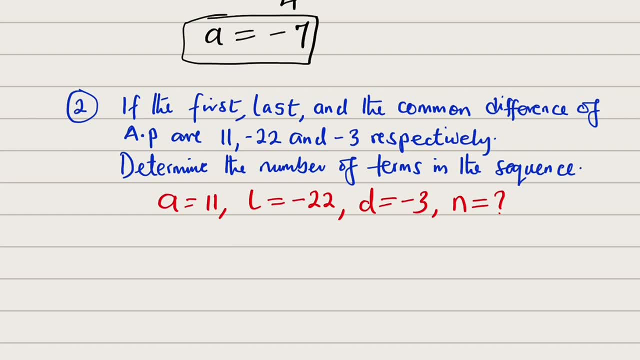 are also asked to find the number of times in this sequence, which is unknown. Remember that the general n-term Tn is equal to a plus n minus 1 multiplied by d. We can use this formula to find the number of times. Let us substitute: 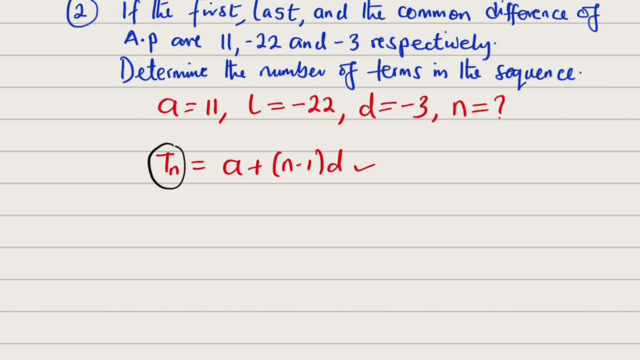 everything here. Tn can serve as any term in a sequence, But since we are given the last term, we can substitute the last term with Tn. Therefore we have negative 22 here, which is equal to A11 plus n minus 1. 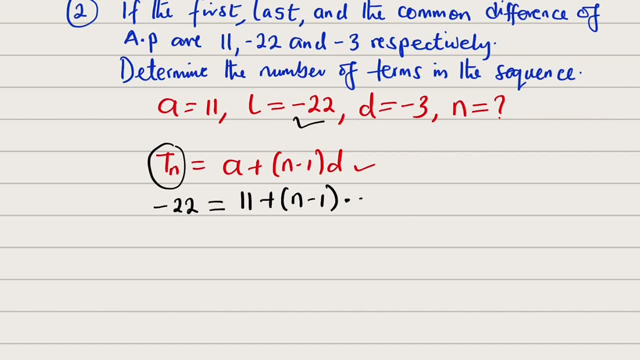 because I have negative 22.. n is still unknown. Multiply by negative 3, which is the constant common difference. Let us use this negative 3 to expand this parenthesis. We have negative 22 to the left, To the right, we have 11.. n multiplied by negative 3 is negative 3n. Negative 1 multiplied by. 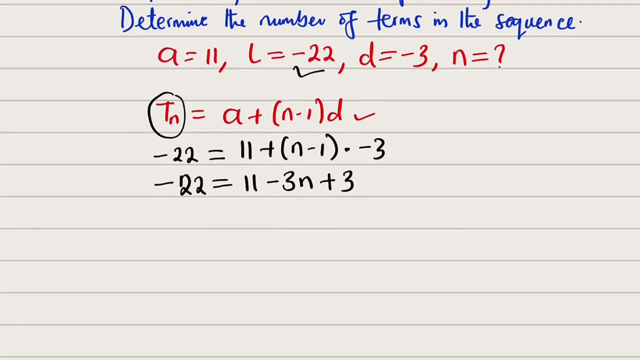 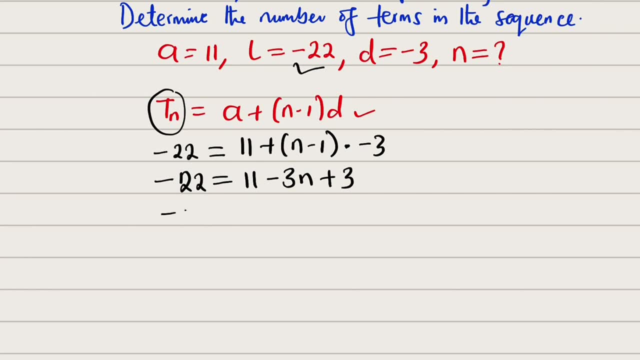 negative 3 is positive 3.. 11 plus 3 is 14.. So we have to the left, 22 negative equals 14 minus 3n. Let us take this 14 to the left. We have negative 22,. negative 14 and this is equal to negative 3n.